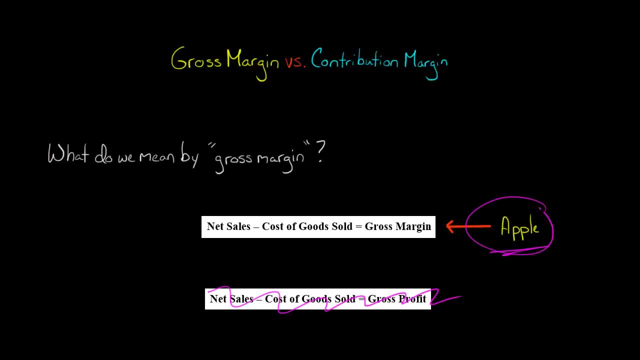 So we're going to ignore that in this video because I'm going to do an example using Apple's actual financial statements. So we're going to take their definition of gross margin, which is net sales minus cost of goods sold, or aka minus cost of sales. 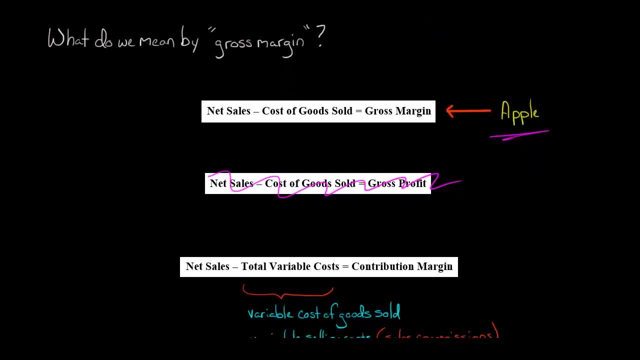 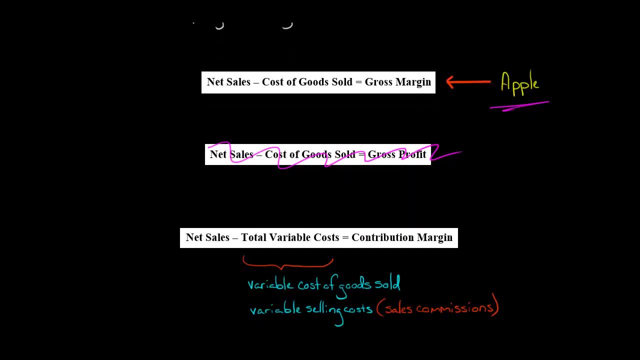 Now, what is contribution margin? Contribution margin is a company's net sales minus its total variable costs. Okay, so contribution margin and the gross margin. in each case, we're starting with a company's net sales, but then we're subtracting something different. 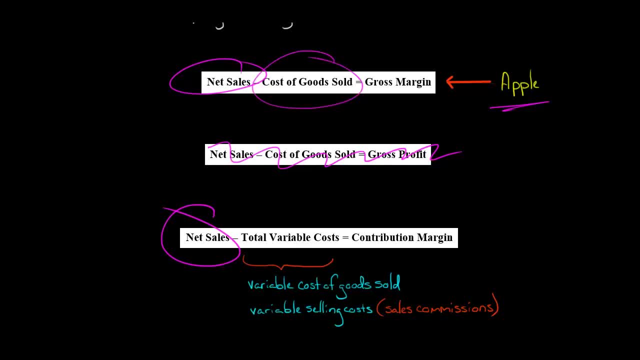 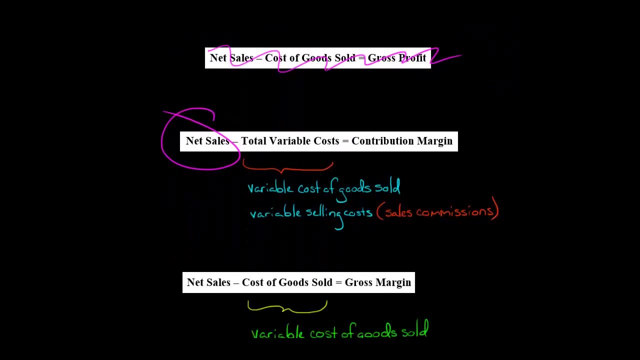 With gross margin, we're subtracting cost of goods sold, and with contribution margin, we are subtracting total variable costs. Now some people will be like: well, what's the difference? Isn't cost of goods sold a variable cost? 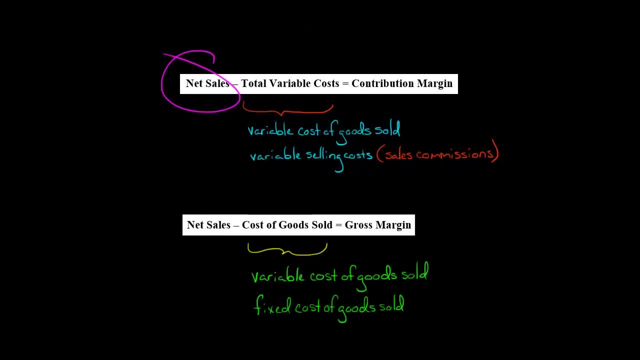 Well, when we look at a manufacturer like Apple, cost of goods sold is going to have a variable and a fixed component. Okay, there's going to be variable costs included in cost of goods sold and fixed costs. And you say: what are the fixed costs that would be included in Apple's cost of sales? 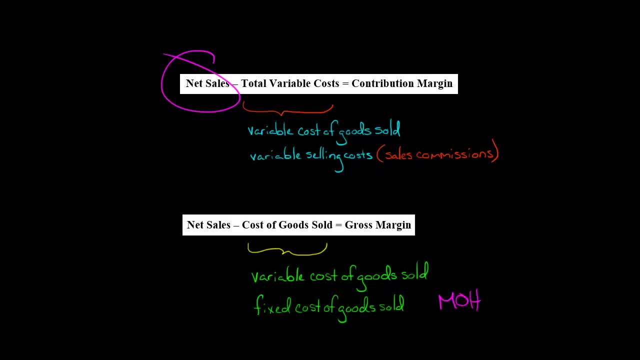 Well, you're going to have manufacturing overhead, And manufacturing overhead has a variable component to it and it has a fixed component to it. Okay, so the fixed component of manufacturing overhead that is ultimately going to be expensed through Apple's cost of goods sold. 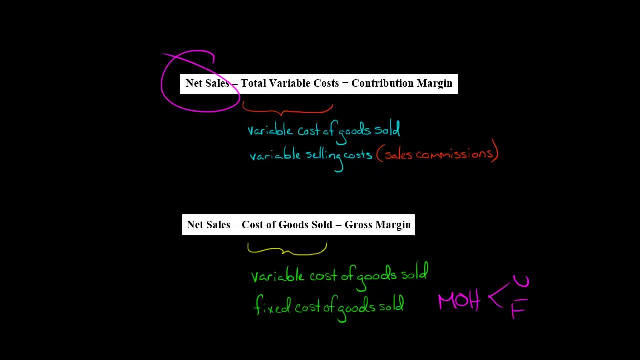 So when you look at Apple's gross margin, which we will in a minute, when you subtract that cost of goods sold, or cost of sales as they refer to it, when you subtract that cost of sales, there are some fixed costs being deducted from net sales to get gross margin. 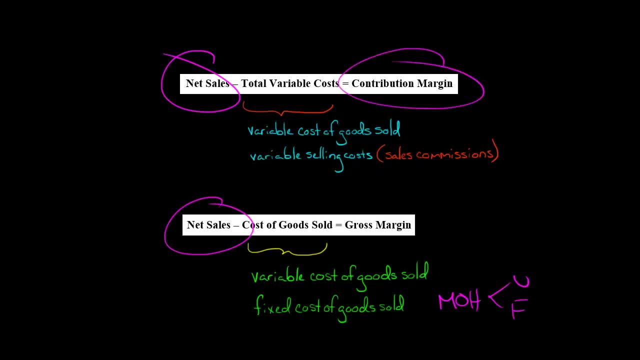 Whereas when we calculate their contribution margin, which I'm going to do using some assumptions, they don't actually present it on their income statement. When you calculate their contribution margin, there are no fixed costs being subtracted. You're just subtracting variable costs from net sales to get contribution margin. 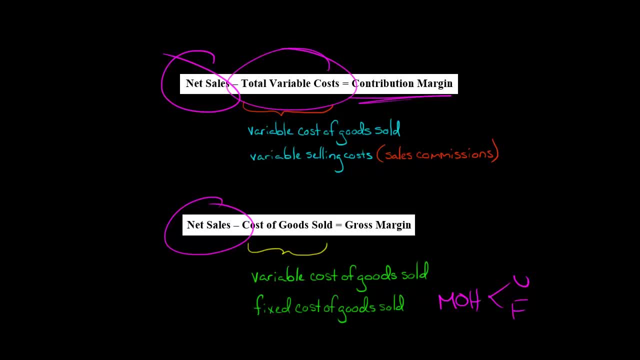 Another difference is here we're subtracting all the variable costs, not just variable costs that have to do with cost of goods sold. So, for example, variable selling costs such as sales commissions would be deducted from net sales and getting. 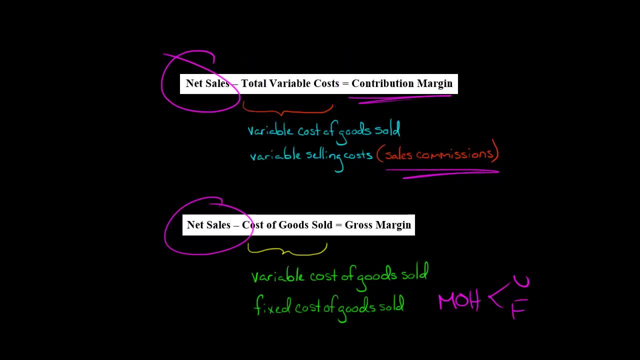 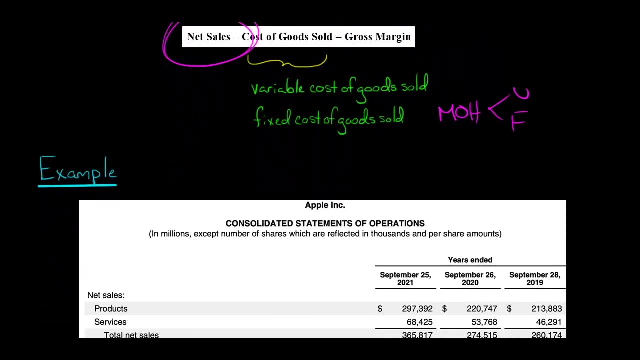 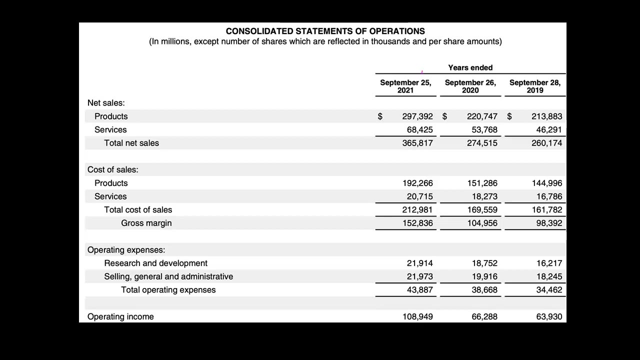 let's say Apple's contribution margin, but you would not subtract sales commissions from net sales in order to get gross margin. So let's look at Apple's actual income statement. We actually have a partial of three different income statements here for the years ended September 25th: 2021, and then 2020, and then 2019.. 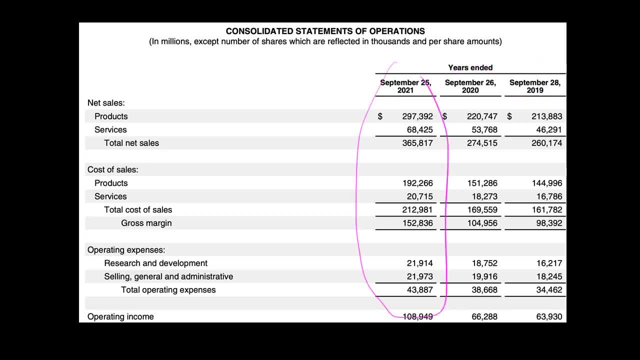 So we're just going to focus on this income statement right here And you can see we've got the total net sales And then the total cost of sales, aka cost of goods sold. So we've got the net sales and you subtract the cost of sales and you get to gross margin right here. 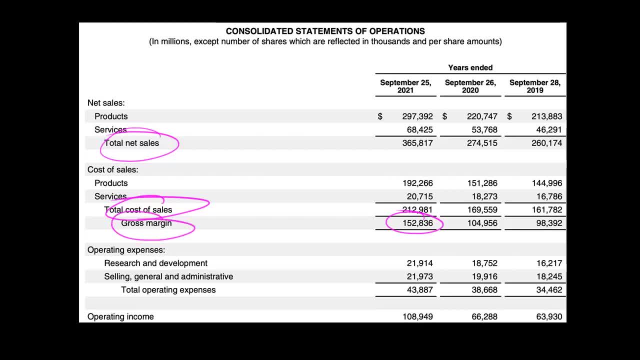 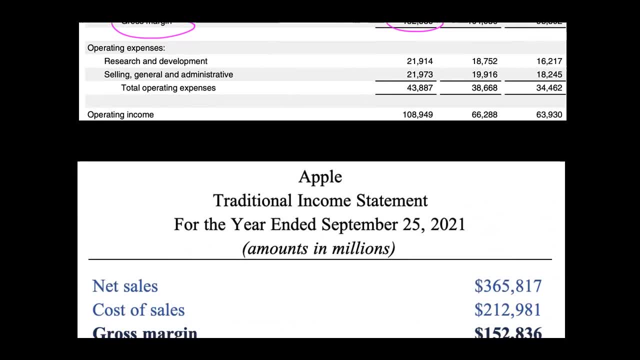 So they had a gross margin of a little over $152 billion, because these amounts are in millions. Now let's break this down. I made a little simpler income statement here So you can see again. this is the same numbers from the income statement we just looked at. 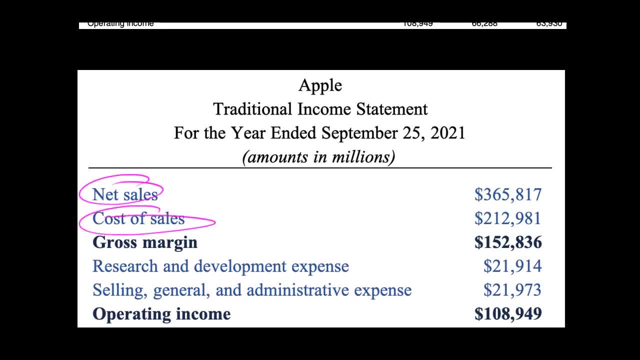 but we've got their net sales minus their cost of sales, aka cost of goods sold, is their gross margin a little over $152 billion. So this cost of sales figure. there's going to be some fixed costs that are in there. 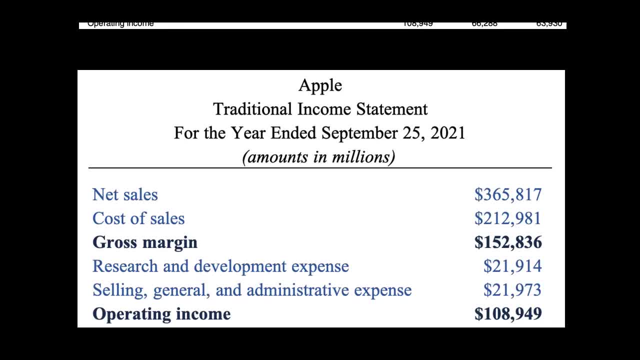 It's not just variable costs that are in that cost of sales. Any fixed manufacturing overhead costs. so fixed manufacturing overhead are going to be a part of that cost of sales. But when you calculate their contribution margin, fixed manufacturing overhead would not be subtracted. 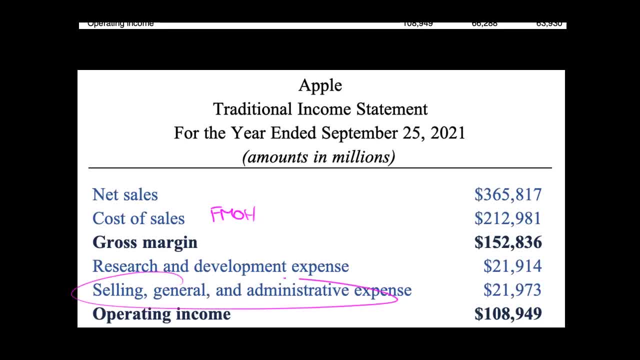 Okay, So here we've got selling general and administrative expense, so we've got some selling costs in here. Let's say that there were some sales commissions that Apple had to pay some of its staff right. So those sales commissions were not deducted to calculate gross margin. 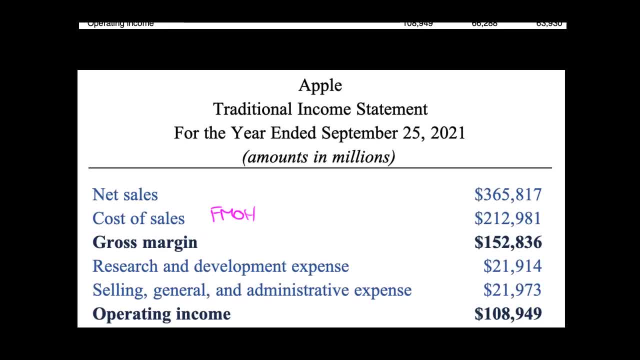 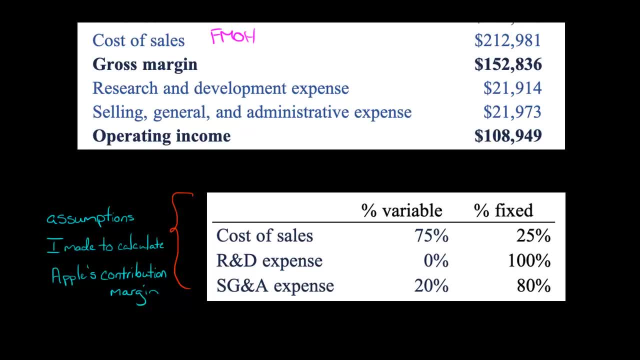 because they are down here after they've already calculated gross margin. So now to calculate, because they didn't actually disclose their contribution margin. I made some assumptions here. We need to make some assumptions about what percentage of each cost is variable, what percentage is fixed. 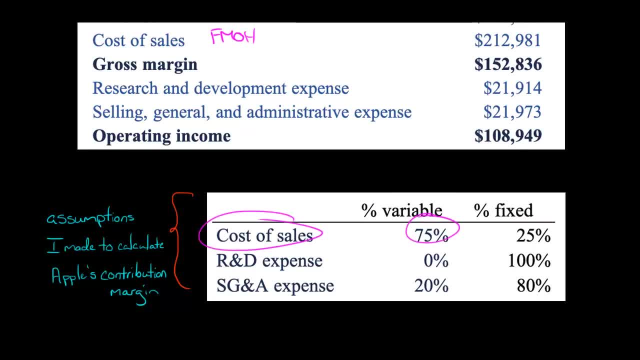 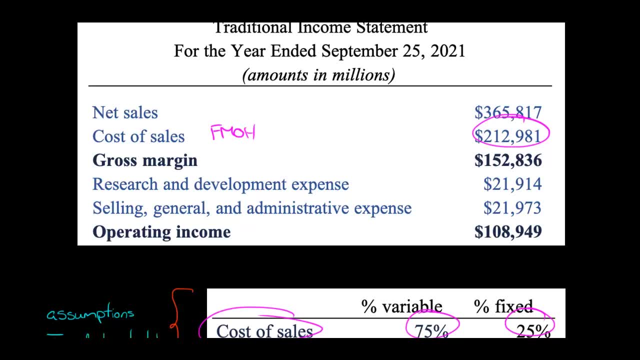 So I'm going to Assume here that the cost of sales is 75% variable, 25% fixed. So if we go back here the cost of sales is a little over $212 billion. I'm going to assume that 25% of that is fixed.